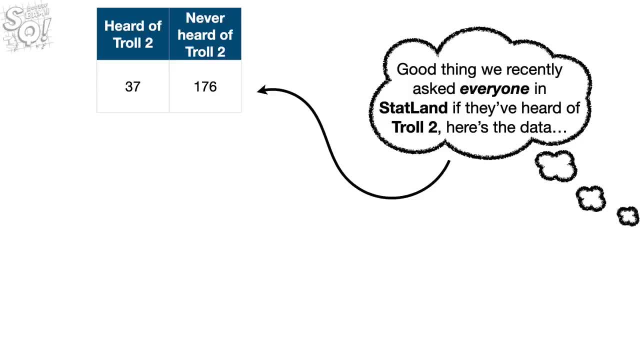 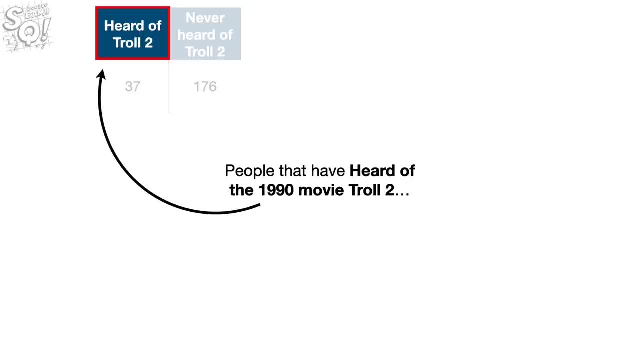 heard of the movie Troll 2.. Here's the data. There are two types of people in Statland: People that have heard of the 1990 movie Troll 2, and people who have never heard of Troll 2.. In other words, there isn't anyone who has both sort of heard of Troll 2 and sort of hasn't heard. 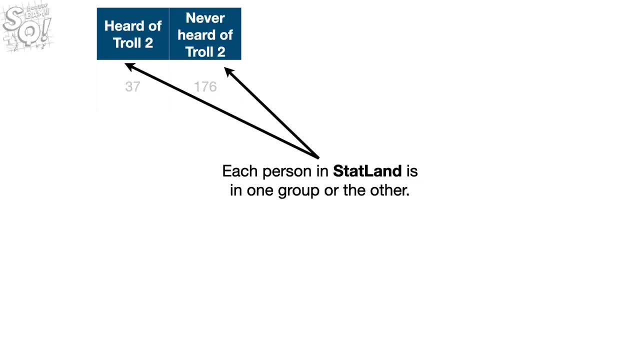 of Troll 2.. Each person in Statland is in one group or the other. 37 of the people in Statland have heard of Troll 2, and the remaining 176 people in Statland have never heard of Troll 2.. That means there are 213 people living in Statland. 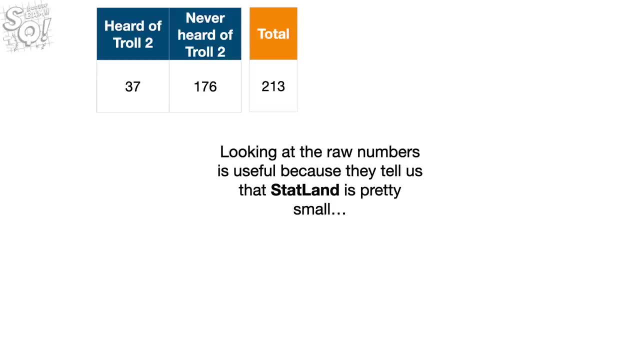 So Statland is not a huge place. Looking at the raw numbers is useful because they tell us that Statland is pretty small and that whatever analysis we do only applies to a handful of people. That said, by looking at the numbers we can get a general sense of the trends in Statland. 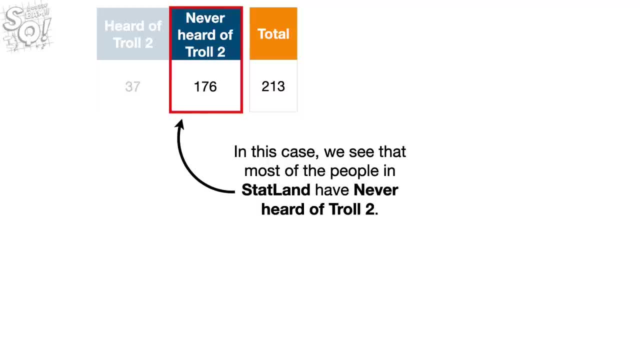 In this case we see that most of the people in Statland have never heard of Troll 2.. But at a glance it's not so bad. It's not super obvious how the number of people who have never heard of Troll 2 relates to the 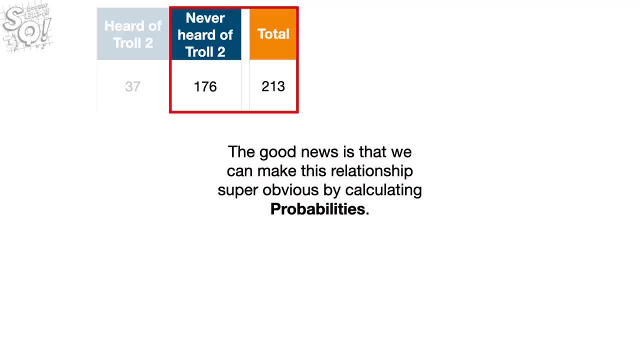 total population of Statland. The good news is that we can make this relationship super obvious by calculating probabilities. So let's calculate the probabilities of people in Statland that have and haven't heard of Troll 2.. If we want to know the probability that a randomly selected 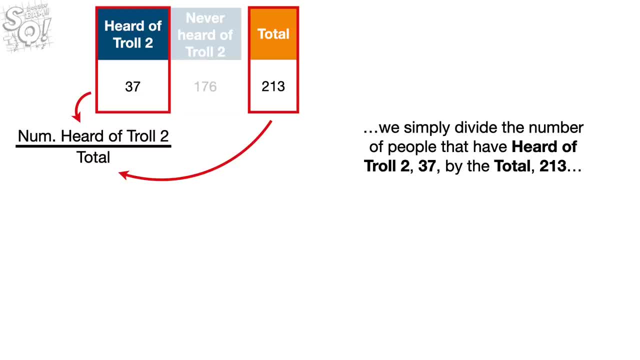 person in Statland has heard of Troll 2,. we simply divide the number of people in Statland by the number of people that have heard of Troll 2,- 37, by the total, 213.. And that gives us 0.17.. 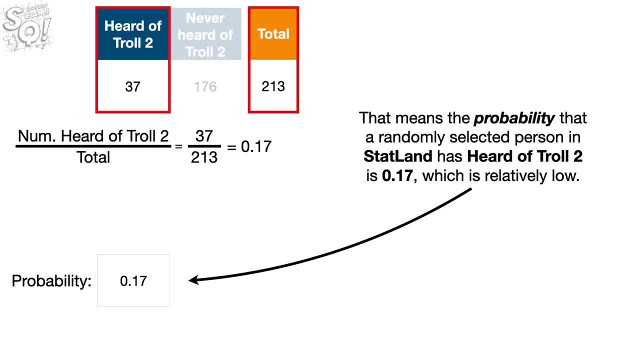 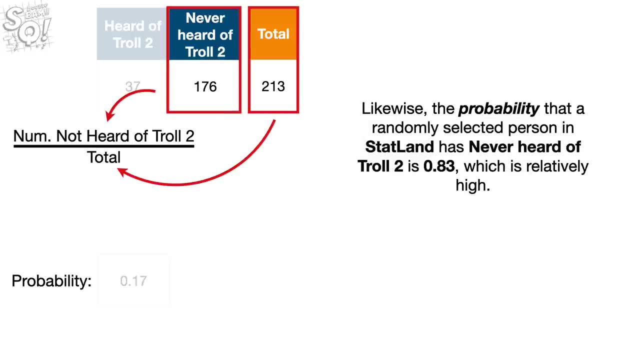 That means the probability that a randomly selected person in Statland has heard of Troll 2 is 0.17,, which is relatively low. Likewise, the probability that a randomly selected person in Statland has never heard of Troll 2 is 0.83,, which is relatively low. 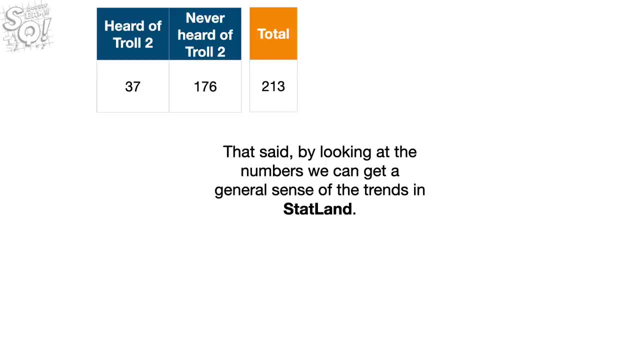 people. That said, by looking at the numbers we can get a general sense of the trends in Statland. In this case we see that most of the people in Statland have never heard of Troll 2.. But at a glance it's not so bad. 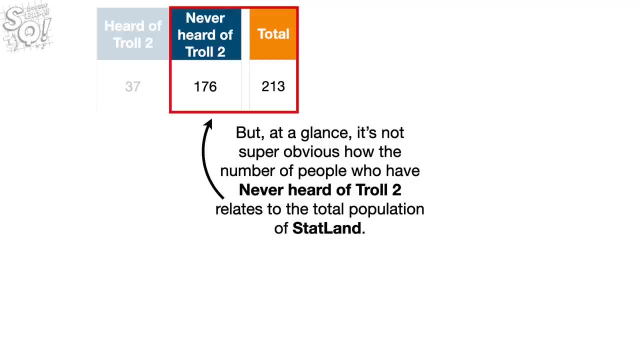 It's not super obvious how the number of people who have never heard of Troll 2 relates to the total population of Statland. The good news is that we can make this relationship super obvious by calculating probabilities. So let's calculate the probabilities of people in Statland that have 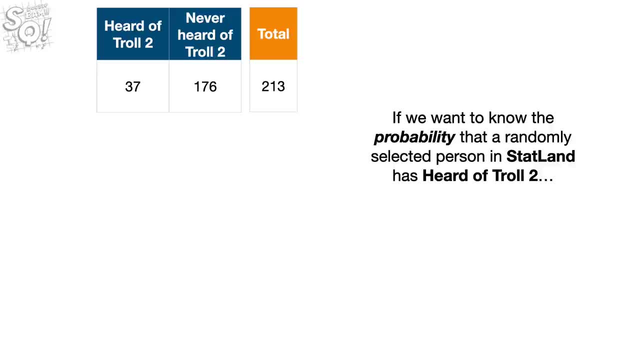 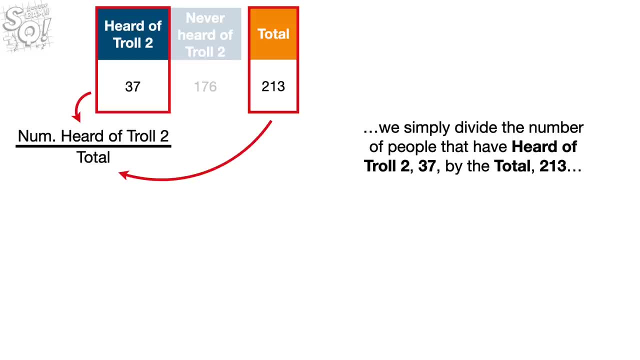 and haven't heard of Troll 2.. If we want to know the probability that a randomly selected person in Statland has heard of Troll 2, we simply divide the number of people in Statland by the number of people that have heard of Troll 2, 37,, by the total: 213.. And that gives us 0.17. 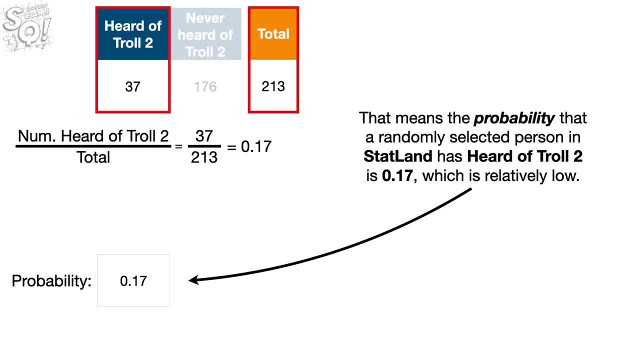 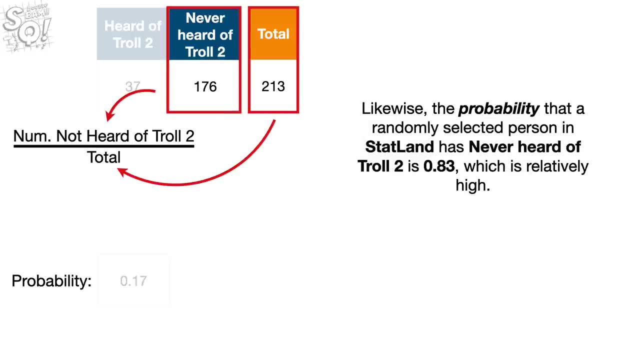 That means the probability that a randomly selected person in Statland has heard of Troll 2 is 0.17,, which is relatively low. Likewise, the probability that a randomly selected person in Statland has never heard of Troll 2 is 0.83,, which is relatively low. 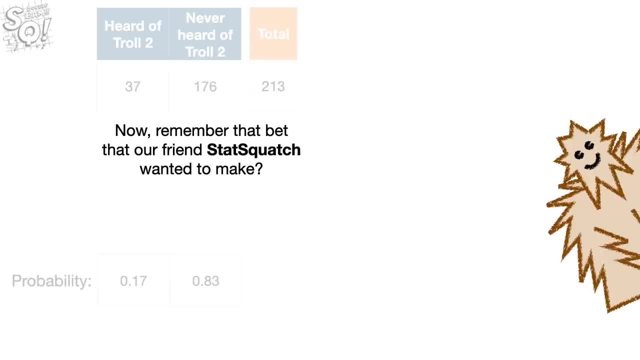 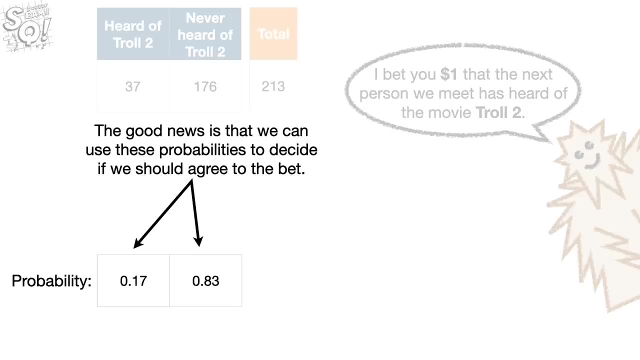 Now remember that bet our friend Statsquatch wanted to make. I bet you $1 that the next person we meet has heard of the movie Troll 2.. The good news is that we can use these probabilities to decide if we should agree to the bet. So let's move the probabilities to the top so we can focus. 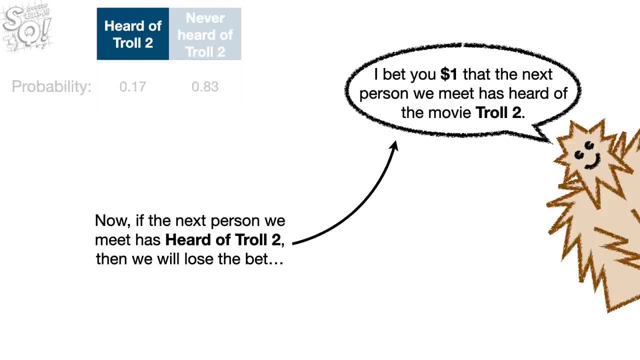 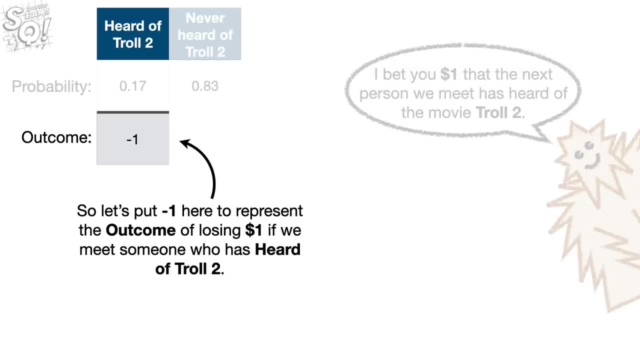 on them. Now, if the next person we meet has heard of Troll 2, then we will lose the bet And that means we will lose $1.. So let's put negative 1 here to represent the outcome of losing $1 if we meet someone who has heard of Troll 2.. In contrast, if the next person has 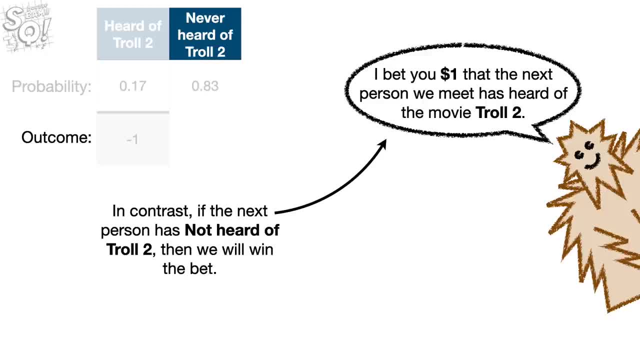 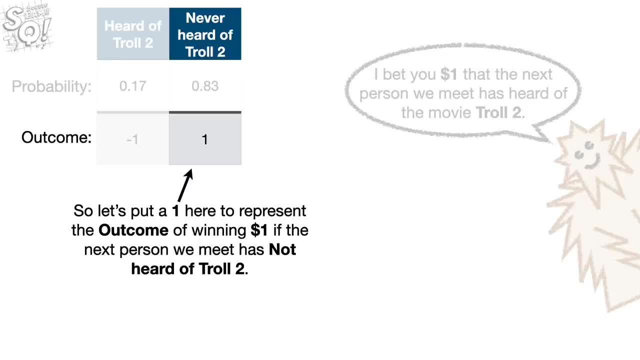 not heard of Troll 2, then we will win the bet And that means we will win $1.. So let's put 1 here to represent the outcome of winning $1 if the next person we meet has not heard of Troll 2.. 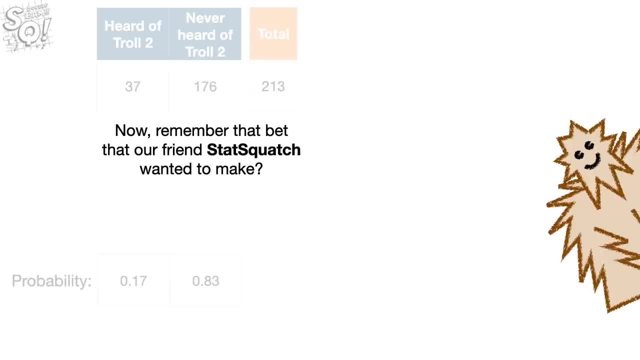 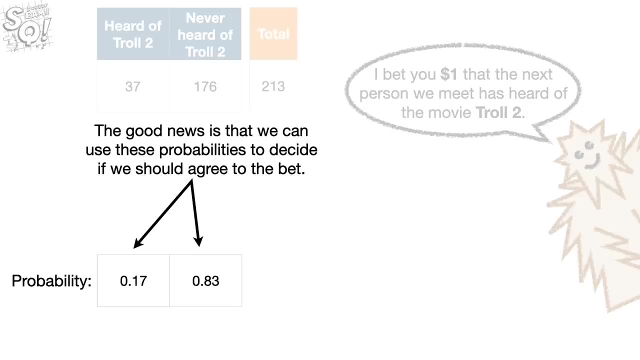 Now remember that bet our friend Statsquatch wanted to make. I bet you $1 that the next person we meet has heard of the movie Troll 2.. The good news is that we can use these probabilities to decide if we should agree to the bet. So let's move the probabilities to the top so we can focus. 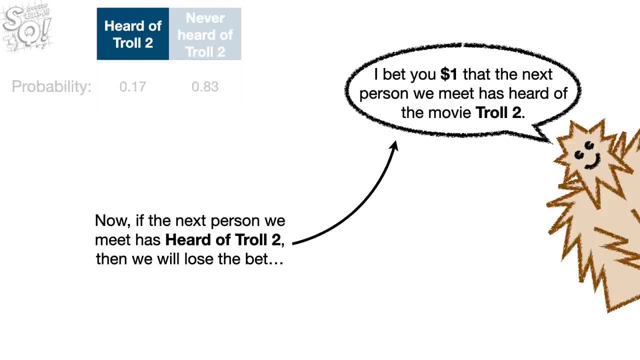 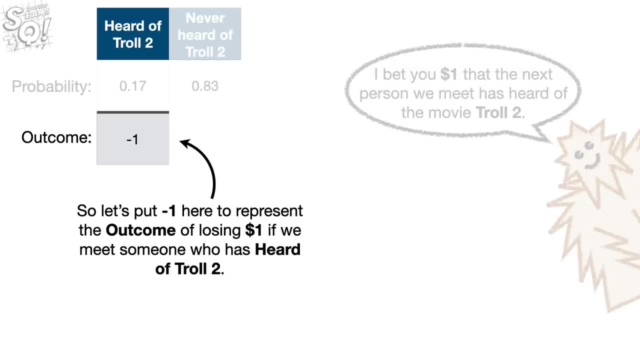 on them. Now, if the next person we meet has heard of Troll 2, then we will lose the bet And that means we will lose $1.. So let's put negative 1 here to represent the outcome of losing $1 if we meet someone who has heard of Troll 2.. In contrast, if the next person has 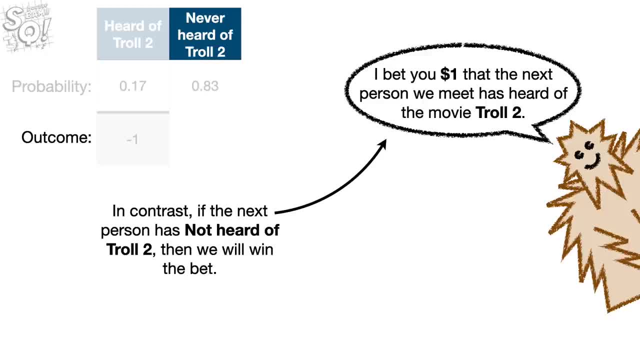 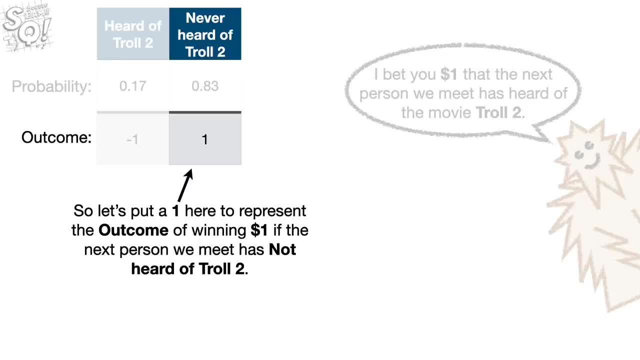 not heard of Troll 2, then we will win the bet And that means we will win $1.. So let's put 1 here to represent the outcome of winning $1 if the next person we meet has not heard of Troll 2.. 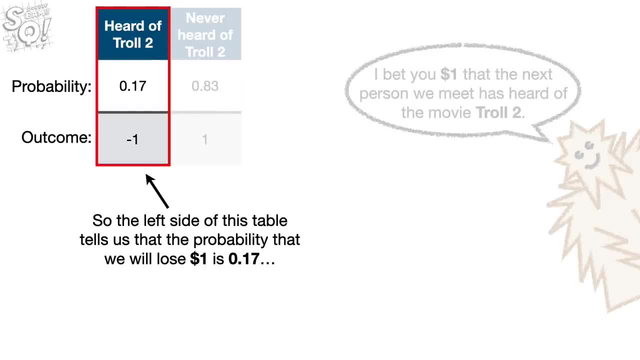 So the left side of this table tells us that the probability we will lose $1 is 0.17.. And the right side tells us that the probability that we will win $1 is 0.83.. In other words, the probability. 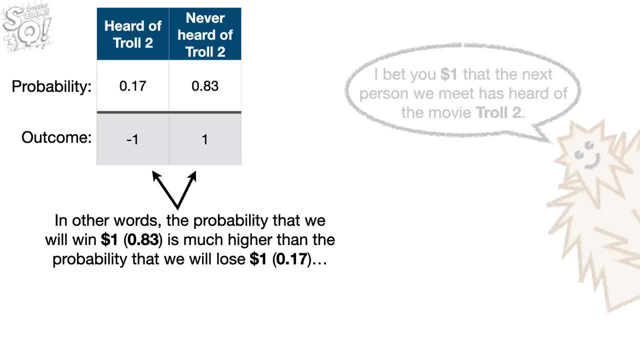 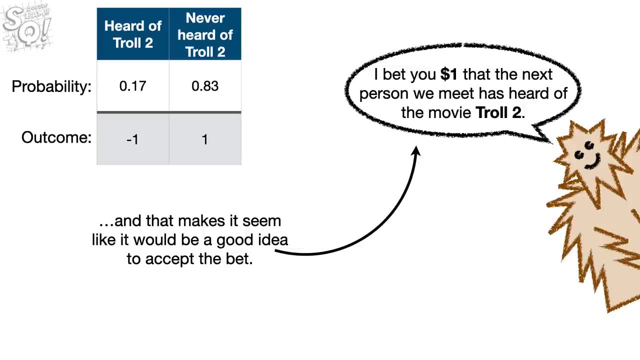 that we will win $1 is much higher than the probability that we will lose $1. And that makes it seem like it would be a good idea to accept the bet. Even though there is a high probability that we will win the bet, there is still a low. 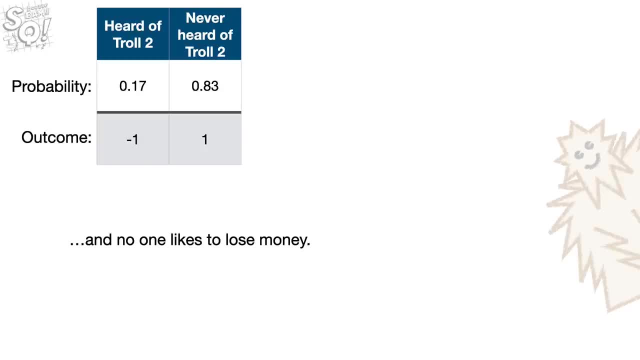 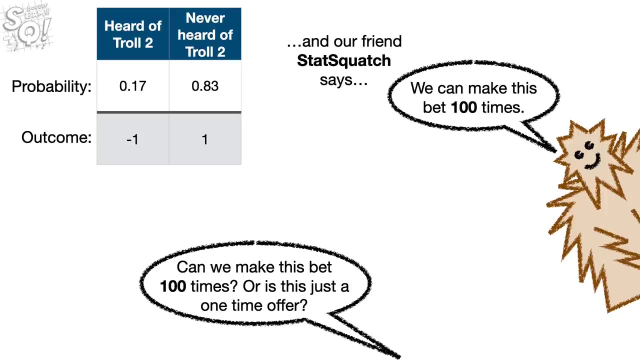 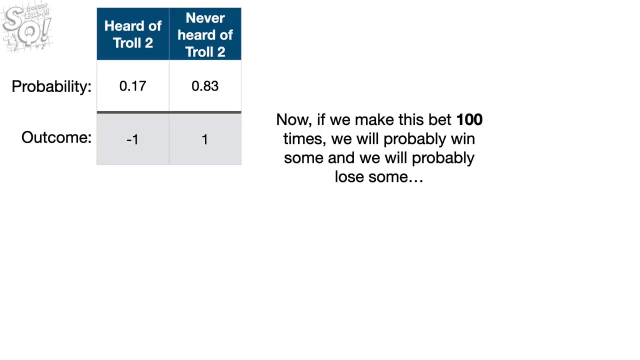 probability that we will lose, And no one likes to lose money. So we say: can we make this bet 100 times or is this just a one-time offer? And our friend Statsquatch says we can make this bet 100 times. Now, if we make this bet 100 times, we will probably win some and we will probably 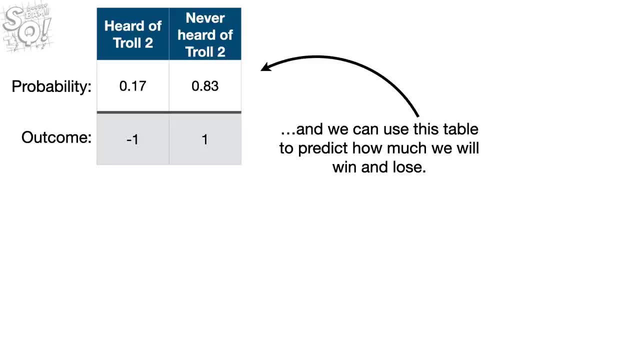 lose some And we can use this table to predict how much we will win and lose. If we make this bet 100 times, we can approximate how many times we will lose by multiplying the probability we will lose 0.17, by 100.. And if we do the math, we get 17.. So that means 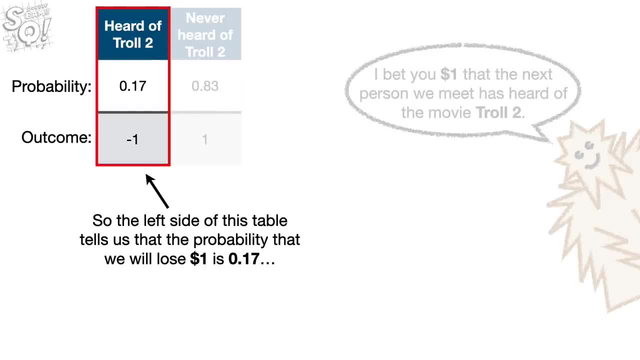 So the left side of this table tells us that the probability we will lose $1 is 0.17.. And the right side tells us that the probability that we will win $1 is 0.83.. In other words, the probability. 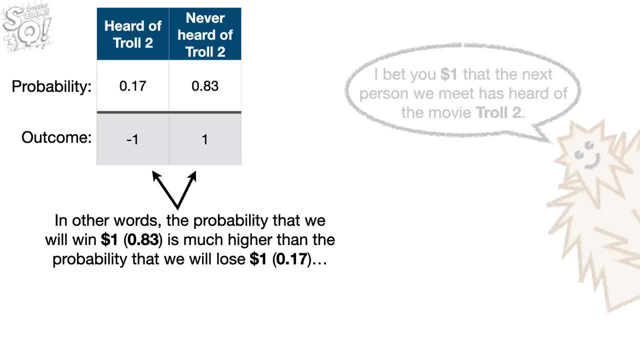 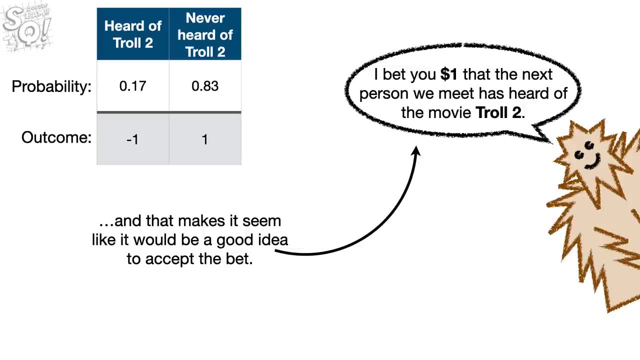 that we will win $1 is much higher than the probability that we will lose $1. And that makes it seem like it would be a good idea to accept the bet. Even though there is a high probability that we will win the bet, there is still a low. 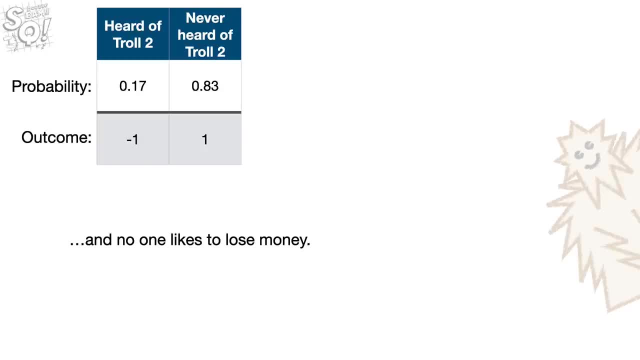 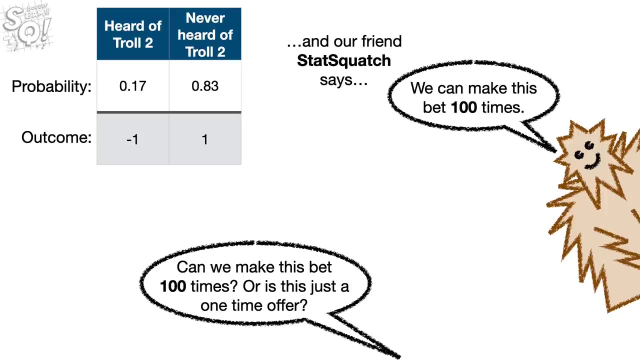 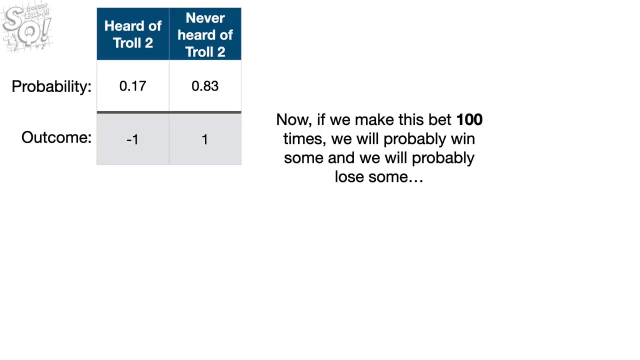 probability that we will lose, And no one likes to lose money. So we say: can we make this bet 100 times or is this just a one-time offer? And our friend Statsquatch says we can make this bet 100 times. Now, if we make this bet 100 times, we will probably win some and we will probably 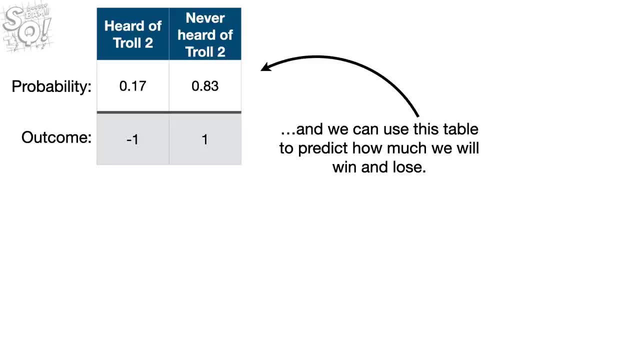 lose some And we can use this table to predict how much we will win and lose. If we make this bet 100 times, we can approximate how many times we will lose by multiplying the probability we will lose 0.17, by 100.. And if we do the math, we get 17.. So that means 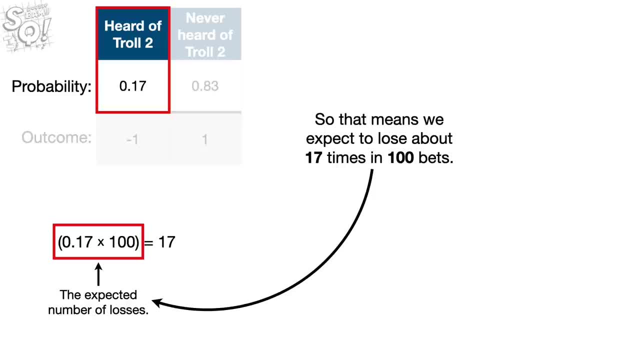 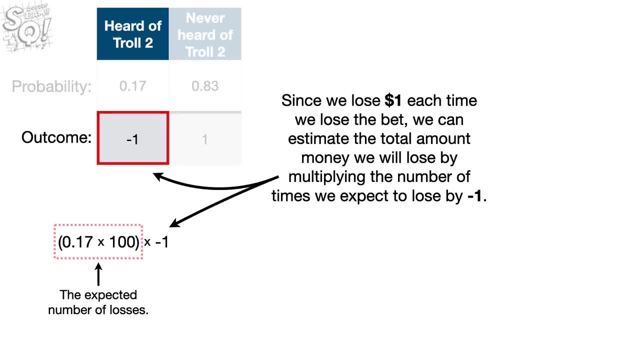 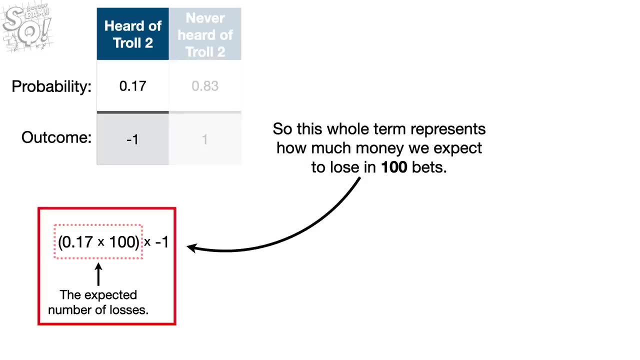 we expect to lose about 17 times in 100 bets. Since we will lose $1 each time we lose $1, we can estimate the total amount of money we will lose by multiplying the number of times we expect to lose by negative 1.. So this whole term represents how much money. 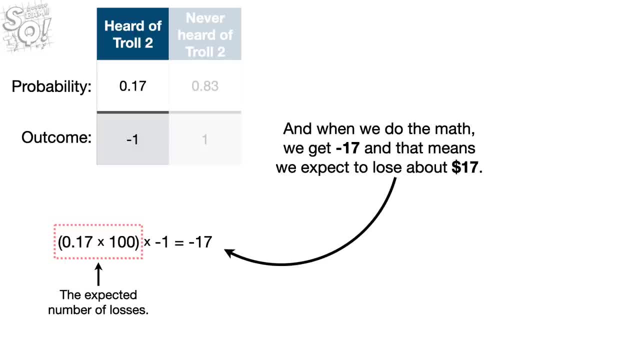 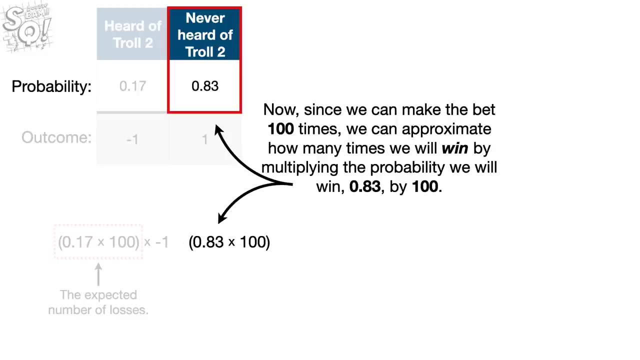 we expect to lose in 100 bets, And when we do the math we get negative 17, and that means we expect to lose about $17.. Wah, wah. Now, since we can make the bet 100 times, we can approximate how many times we will win by multiplying the probability we will. 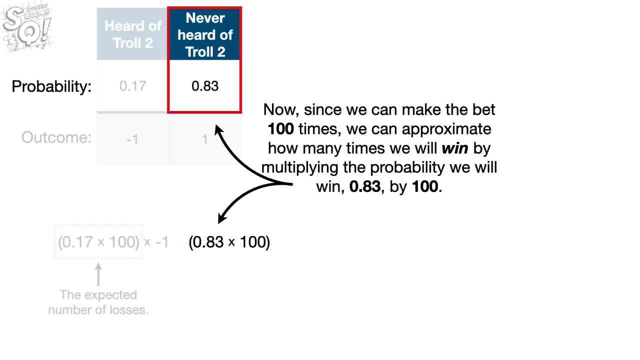 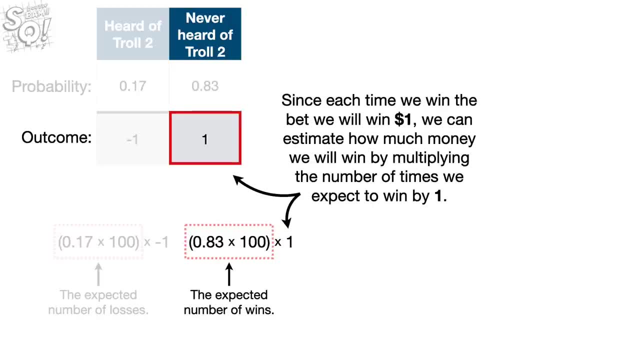 win 0.83, by 100.. When we do the math, we see that we expect to win about 83 times. Since each time we win the bet we will win $1, we can estimate how much money we will. 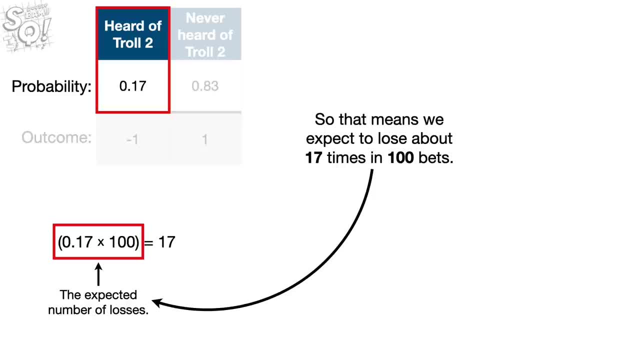 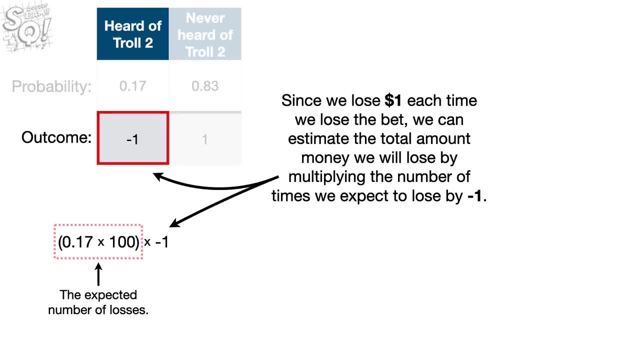 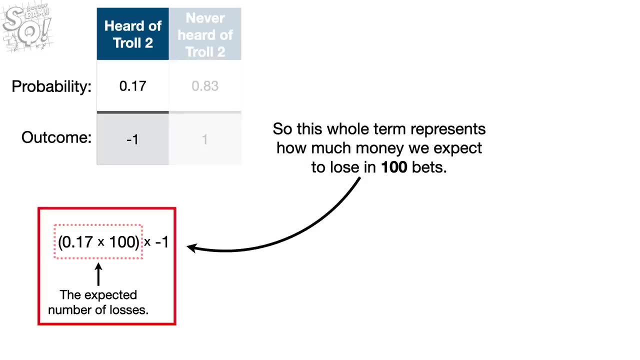 we expect to lose about 17 times in 100 bets. Since we will lose $1 each time we lose $1, we can estimate the total amount of money we will lose by multiplying the number of times we expect to lose by negative 1.. So this whole term represents how much money. 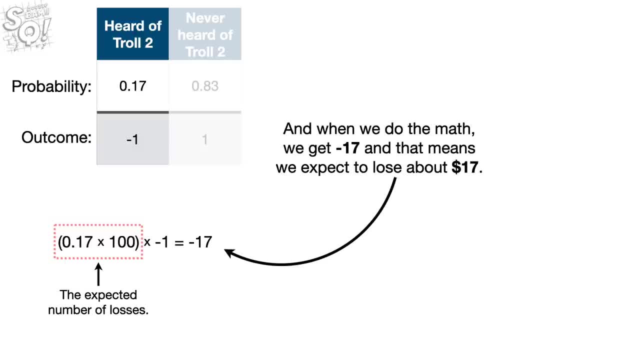 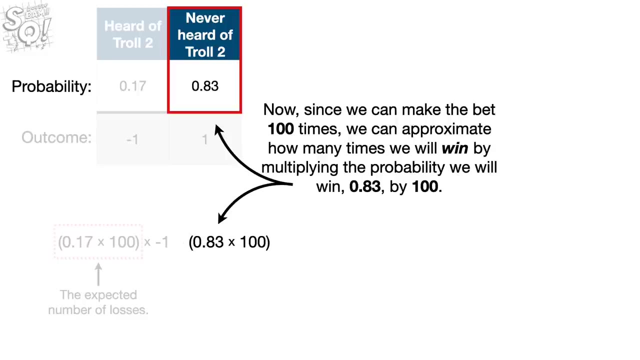 we expect to lose in 100 bets, And when we do the math we get negative 17, and that means we expect to lose about $17.. Wah, wah. Now, since we can make the bet 100 times, we can approximate how many times we will win by multiplying the probability we will. 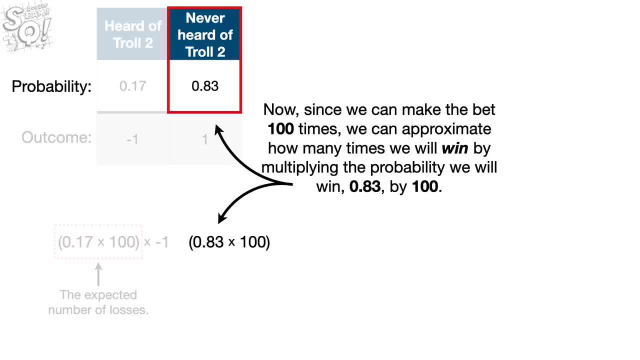 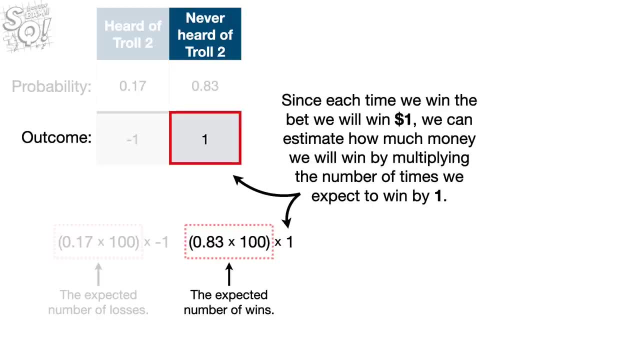 win 0.83, by 100.. When we do the math, we see that we expect to win about 83 times. Since each time we win the bet we will win $1, we can estimate how much money we will. 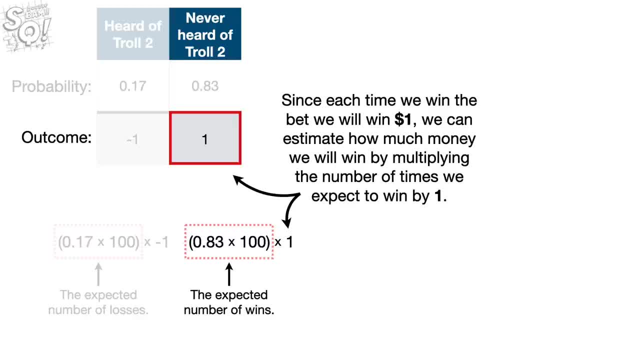 win by multiplying the number of times we expect to win by 1.. So this whole term represents how much money we expect to win by 1.. So that means we can estimate how many times we will win by 100. And if we do the math we see that we expect to win about 83 times, Since each 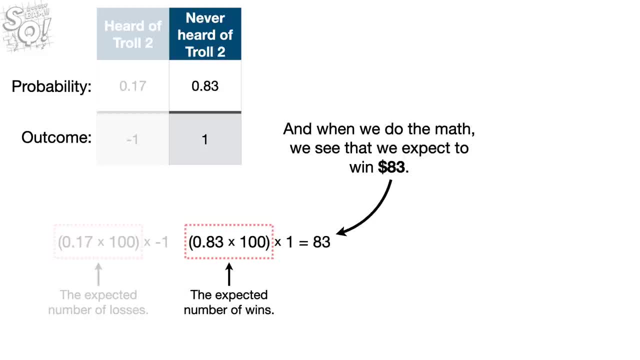 time there is so much money, we expect to win by 100, so this whole term is basically the whole term for how much we wild bet at the playoff. Now that we have a term for the expected amount lost and a term for expected amount won, we can add these two terms to. 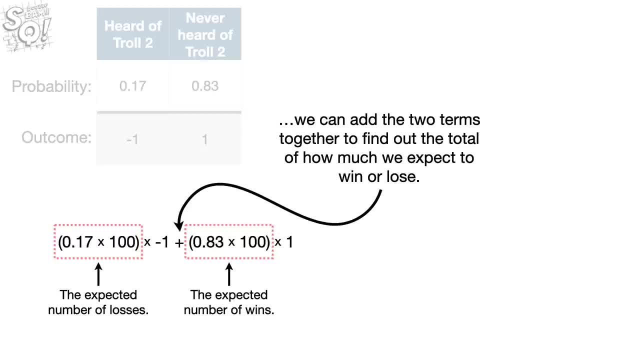 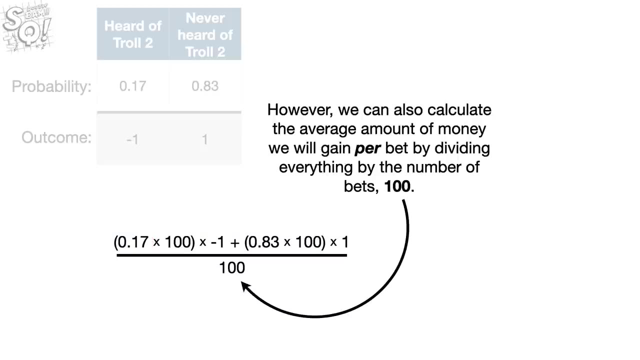 win a bet And when we do the math, we see that we expect to win approximately $66 times $66 after 100 bets. However, we can also calculate the average amount of money we will gain per bet by dividing everything by the number of bets- 100. 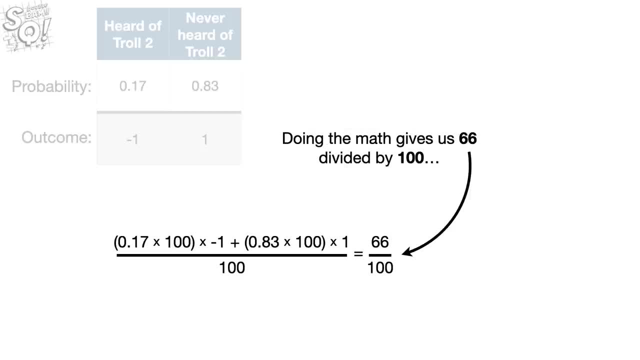 Doing the math gives us 66 divided by 100, which is 0.66.. So on average, we expect to gain 66 cents every time we bet. Note: even though I win or lose $1 each time I bet. 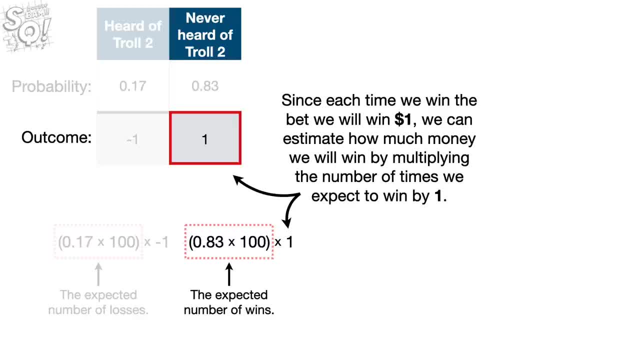 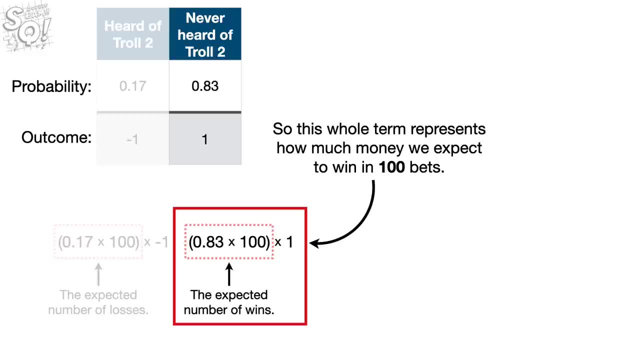 win by multiplying the number of times we expect to win by 1.. So this whole term represents how much money we expect to win by 1. And we can estimate how much money we will win in 100 bets. And when we do the math we see that we expect to win $83.. Now that we have a term for 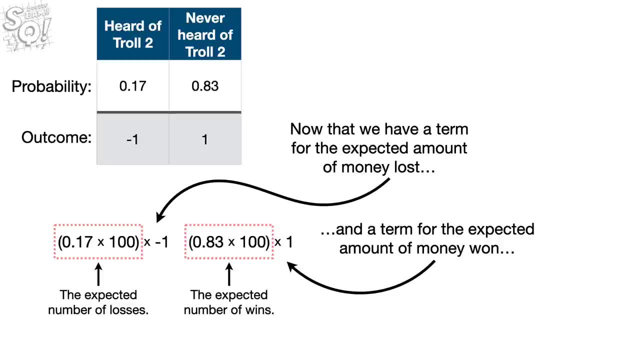 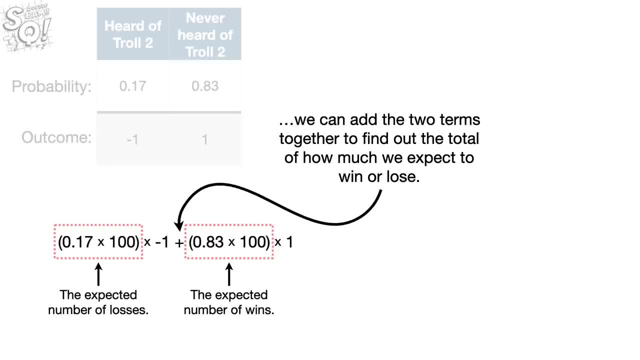 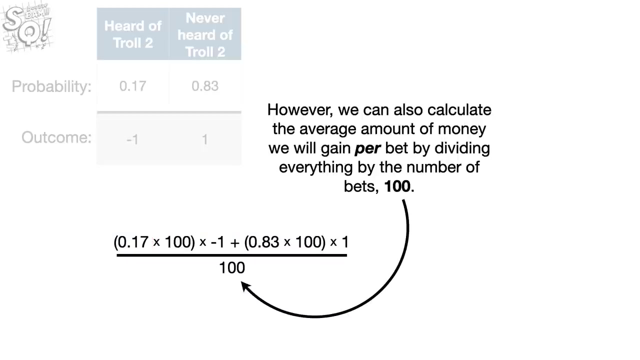 the expected amount of money lost and a term for the expected amount of money won. we can add the two terms together to find out the total of how much we expect to win or lose, And when we do the math, we see that we expect to gain approximately $66 after 100 bets. However, we can also calculate 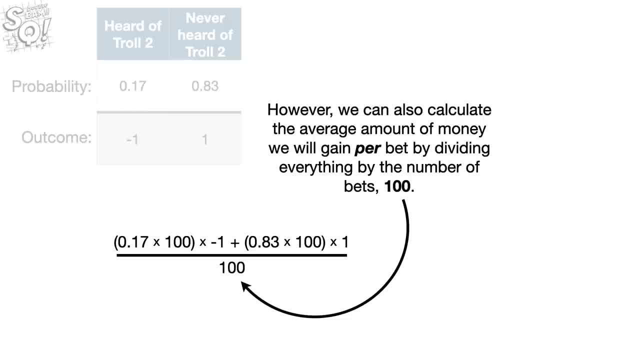 the average amount of money we will gain per bet by dividing everything by the number of bets- 100.. Doing the math gives us 66 divided by 100, which is 0.66.. So, on average, we expect to gain 66 cents every time we bet. 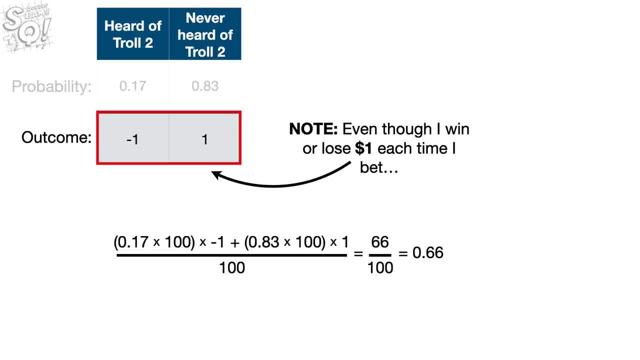 Note: even though I win or lose $1 each time I bet, on average I expect to gain 66 cents each time. In statistics lingo, 66 cents is the expected value for the bet Bam. Using fancy statistics notation, we could write: E of bet equals 0.66. 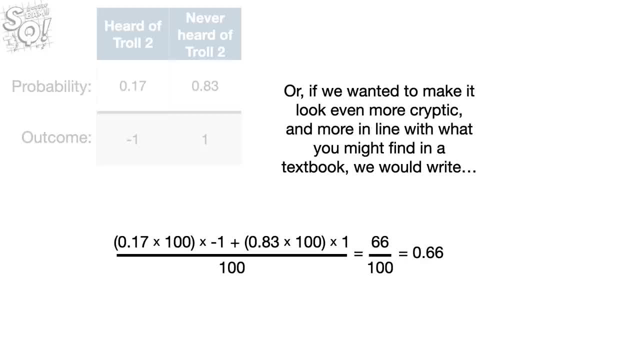 Or if we wanted to make it look even more cryptic and more in line with what you might find in a textbook, we could write: E of x equals 0.66, where x represents the bet. Now let's talk about why I left this messy math in the middle of everything. 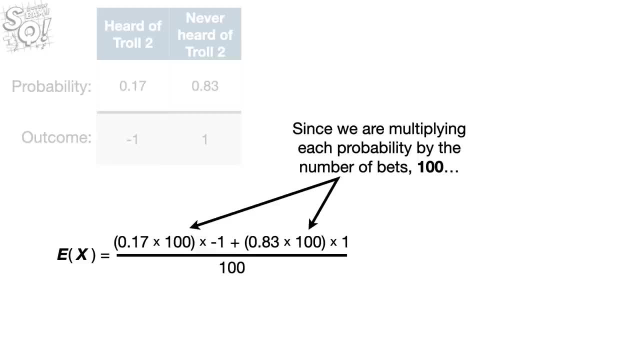 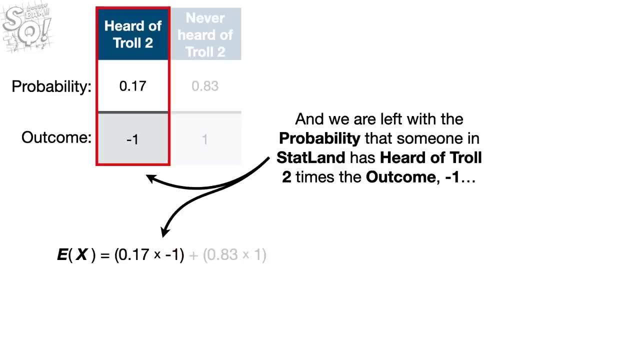 Since we are multiplying each probability by the number of bets 100, and dividing by the number of bets 100,, then all of the values that represent the number of bets 100, cancel out And we're left with the probability that someone in Statland has heard of Troll 2. 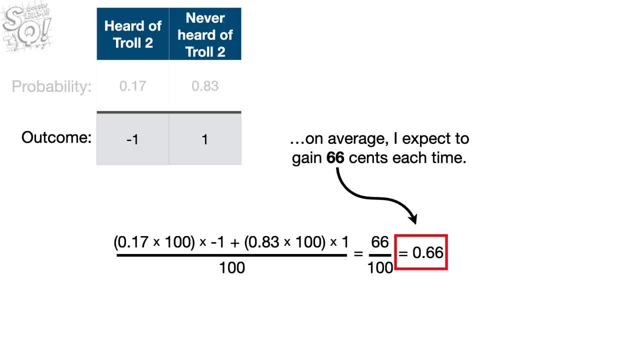 on average, I expect to gain 66 cents each time. In statistics lingo, 66 cents is the expected value for the bet. Bam. Using fancy statistics notation, we could write: E of bet equals 0.66.. Or if we wanted to make it look even more cryptic, 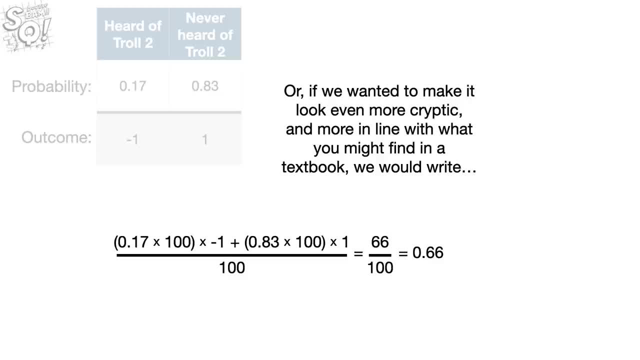 and more in line with what you might find in a textbook. we could write: E of x equals 0.66, where x represents the bet. Now let's talk about why I left this messy math in the middle of everything, Since we are multiplying each probability by the number of bets- 100,. 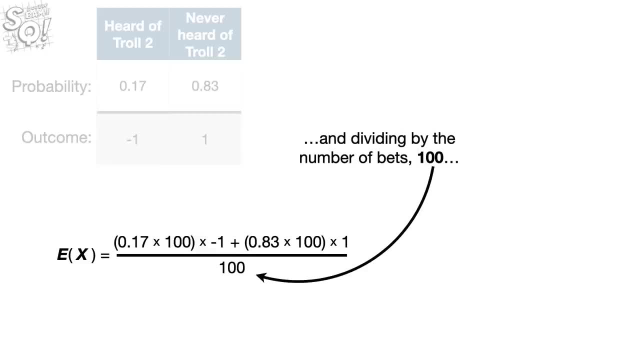 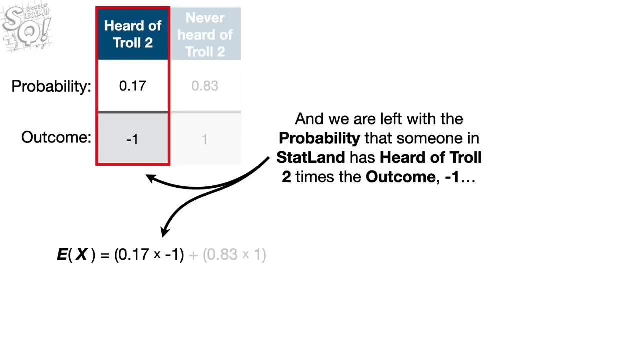 and dividing by the number of bets, then all of the values that represent the number of bets- 100,, cancel out And we're left with the probability that someone in Statland has heard of Troll 2 times the outcome: negative: 1,. 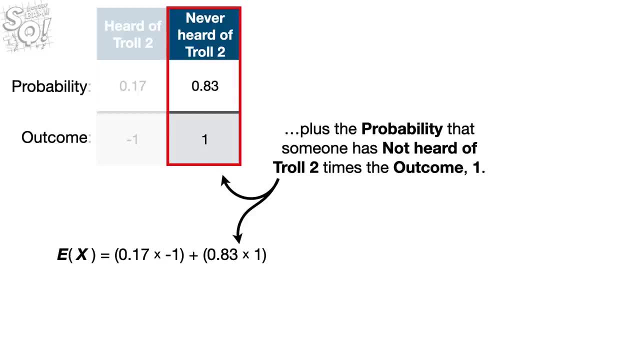 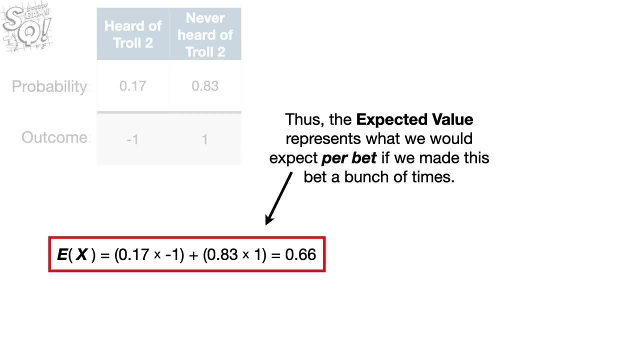 plus the probability that someone has not heard of Troll, 2 times the outcome, 1.. And when we do the math we get the exact same thing we got before: 0.66.. Thus the expected value represents what we would expect per bet. 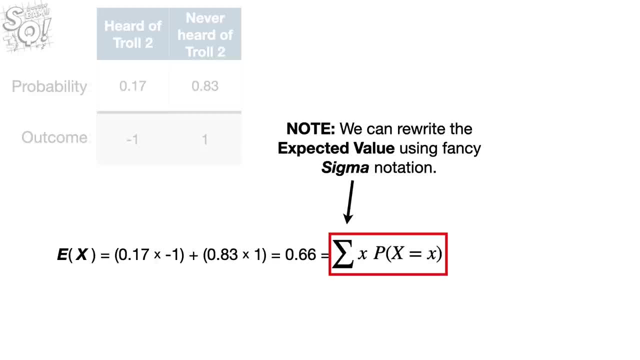 if we made this bet a bunch of times. Note: we can rewrite the expected value using fancy sigma notation. Using fancy sigma notation, the expected value E of x is the sum of each outcome x times the probability of observing each outcome x. 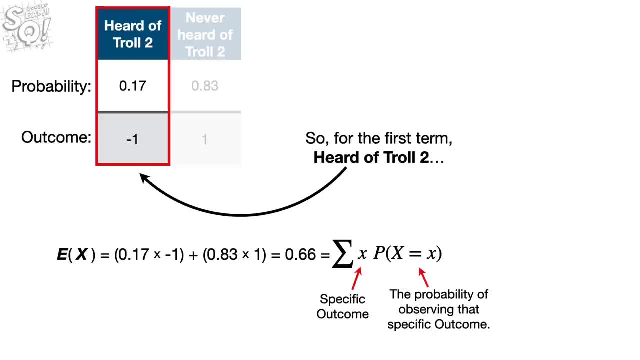 So for the first term heard of Troll 2, the outcome is negative: 1.. And the probability of observing the outcome is 0.17.. So we multiply those values together, then the sigma tells us to add that term to the term for not heard of Troll 2.. 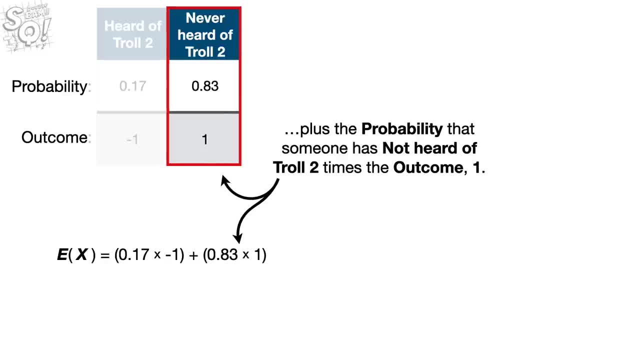 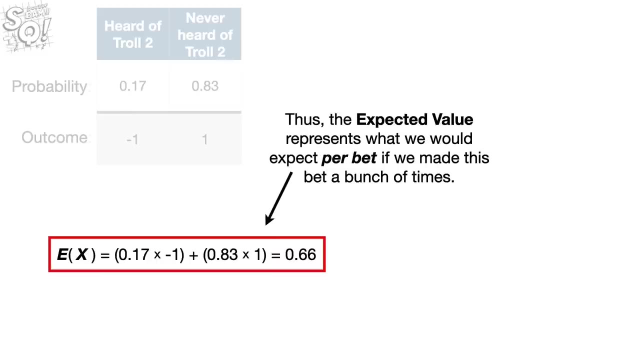 times the outcome negative: 1, plus the probability that someone has not heard of Troll, 2 times the outcome: 1.. And when we do the math we get the exact same thing we got before: 0.66.. Thus the expected value represents what we would expect per bet if we made this bet a bunch of times. 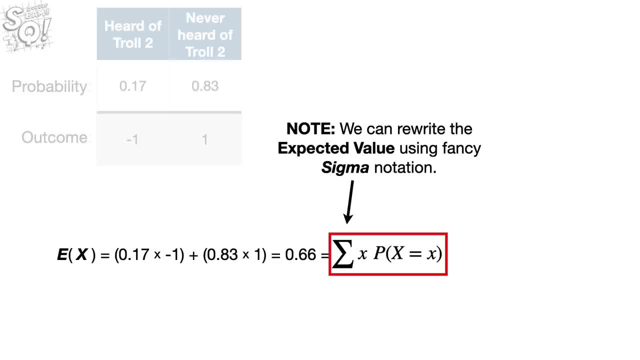 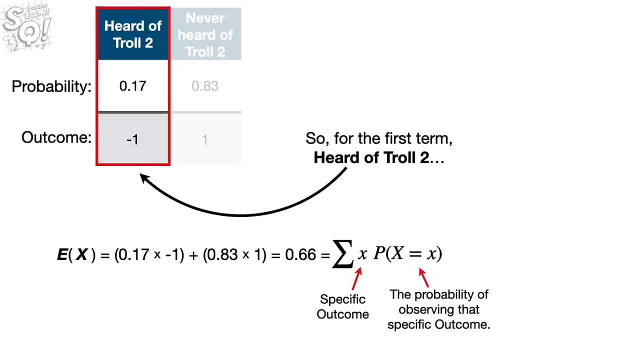 Note: we can rewrite the expected value using fancy sigma notation. Using fancy sigma notation, the expected value E of x is the sum of each outcome x times the probability of observing each outcome, x. So for the first term heard of Troll 2,, the outcome is negative, 1, and the probability of observing 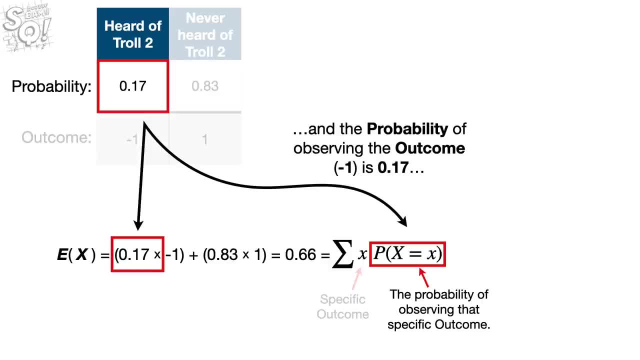 the outcome is 0.17.. So we multiply those values together, Then the sigma tells us to add that term to the term for not heard of Troll, 2.. Now the outcome is 1, and the probability of observing the outcome is 0.18.. 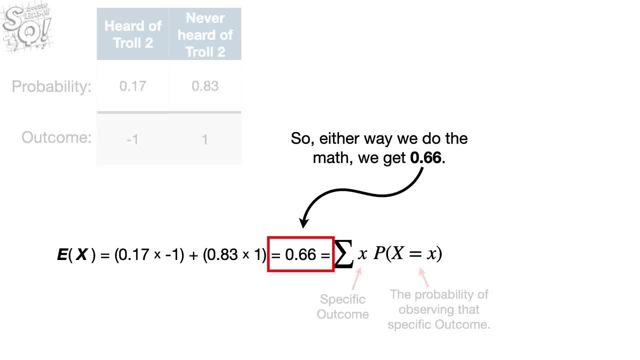 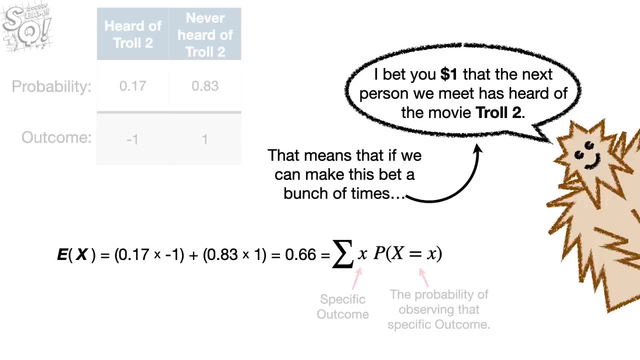 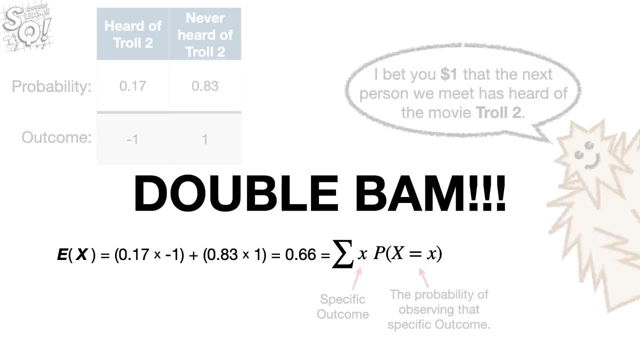 So either way we do the math, we get 0.66.. That means that if we can make this bet a bunch of times, even though we will lose some of the time, we should make money in the long run. Double bam. 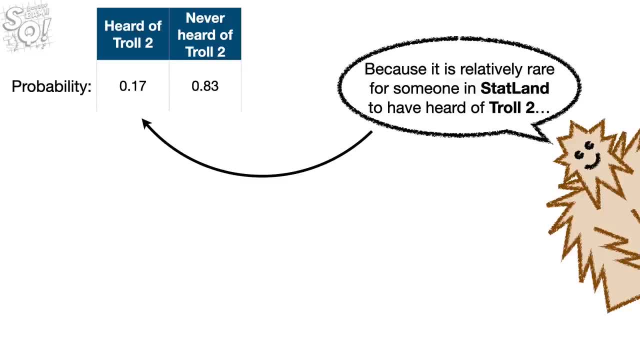 Now imagine StatSquatch saying: because it is relatively rare for someone in Statland to have heard of Troll 2, I will pay you $10.00.. That is if the next person we meet has heard of Troll 2, but if they have not, you pay me. 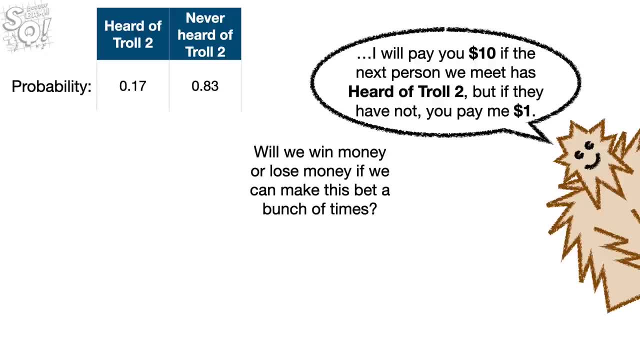 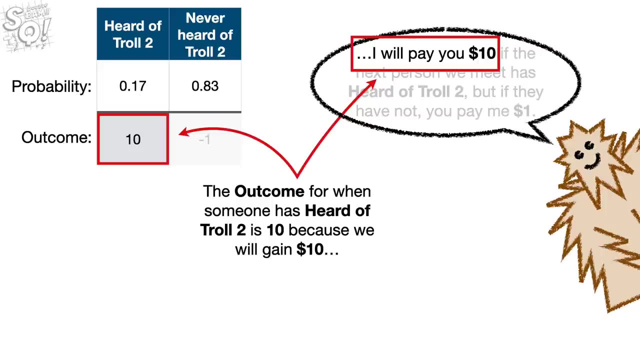 $1.00.. Will we win money or lose money if we can make this bet a bunch of times? Let's calculate the expected value to find out The outcome. for when someone has heard of Troll 2 is 10, because we will gain $10.00. 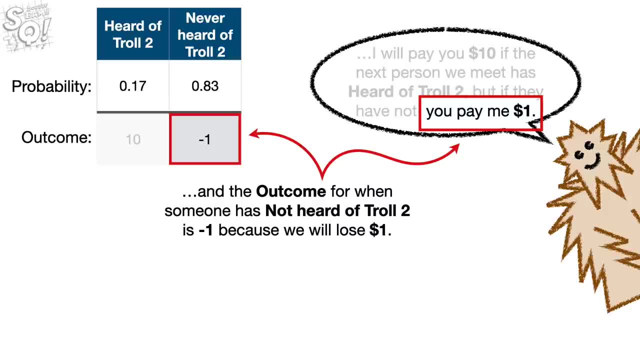 And the outcome for when someone has not heard of Troll 2 is negative 1, because we will gain $10.00.. And the outcome for when someone has not heard of Troll 2 is negative 1, because we will lose $1.00.. 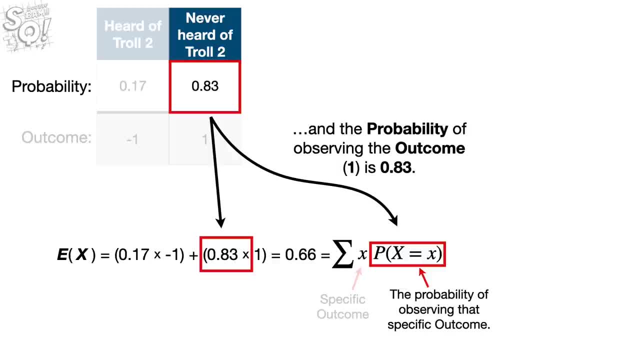 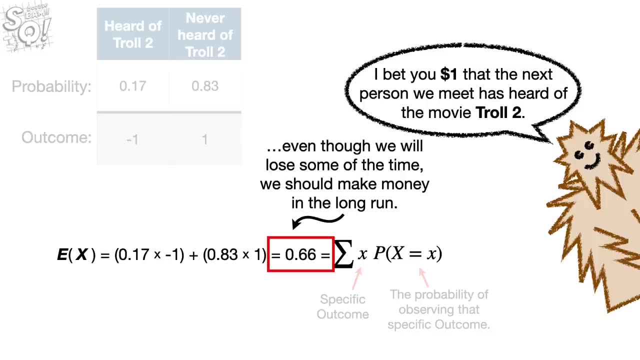 Now the outcome is 1, and the probability of observing the outcome is negative. 1. is 0.83.. So either way we do the math, we get 0.66.. That means that if we can make this bet a bunch of times, even though we will lose some of the time, we should make money. 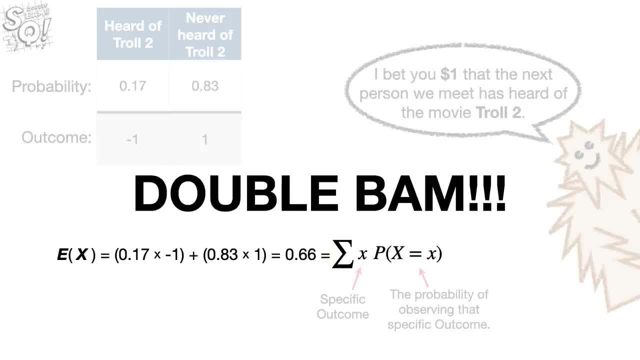 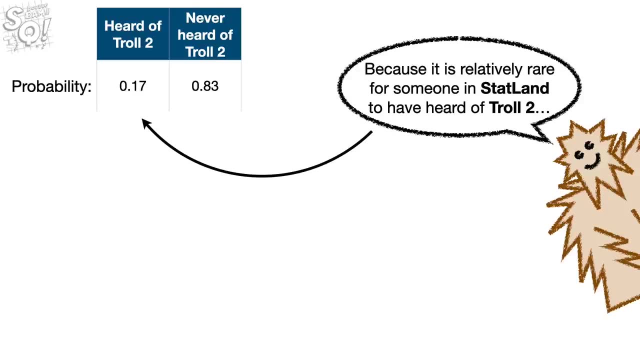 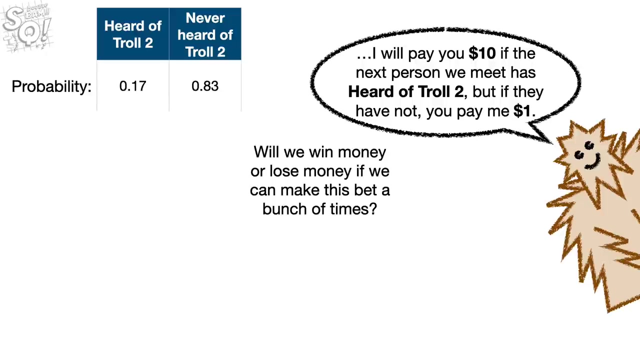 in the long run. Double bam. Now imagine Statsquatch saying: because it is relatively rare for someone in Statland to have heard of Troll 2, I will pay you $10 if the next person we meet has heard of Troll 2, but if they have not, you pay me $1.. Will we win money or lose? 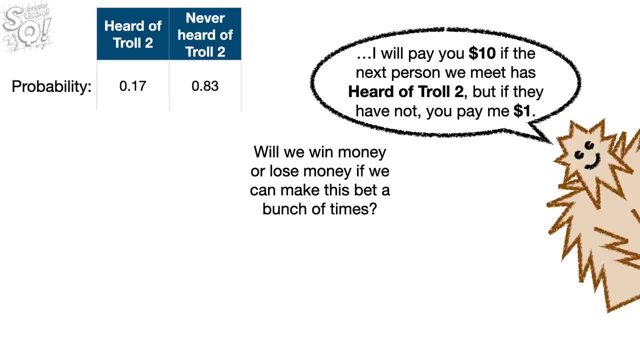 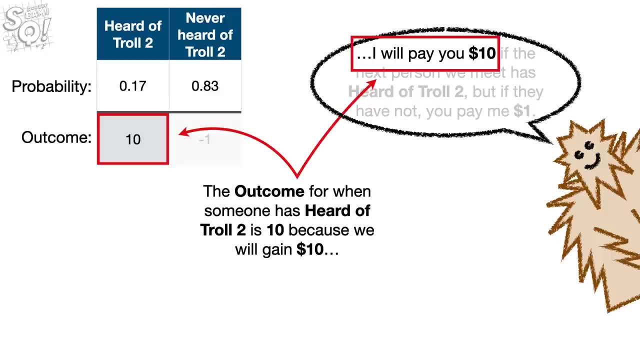 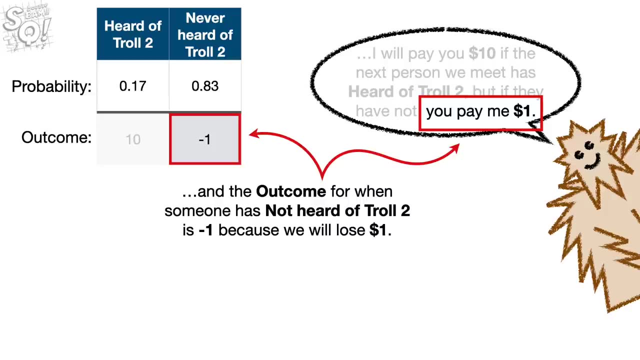 money if we can make this bet a bunch of times. Let's calculate the expected value to find out. The outcome for when someone has heard of Troll 2 is 10, because we will gain $10.. And the outcome for when someone has not heard of Troll 2 is negative- 1, because we will lose. 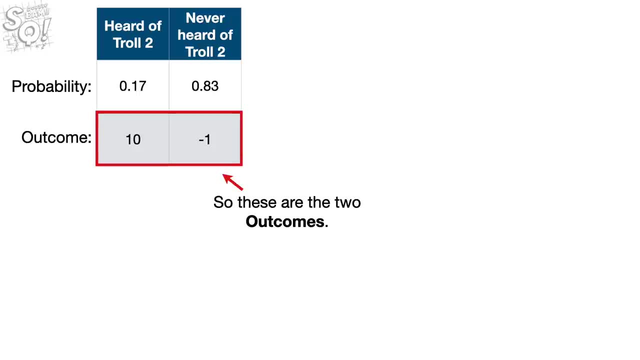 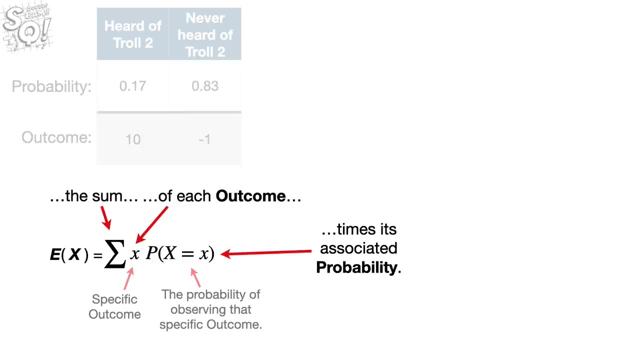 $1.. So these are the two outcomes. Now let's calculate the expected value. The expected value is the sum of each outcome times its associated probability. So let's start by plugging in the numbers. for heard of Troll 2.. 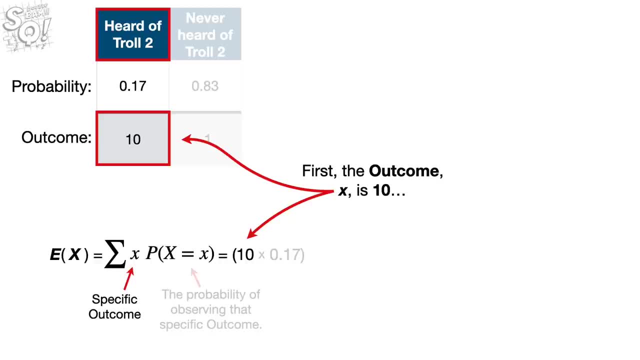 First, the outcome x is 10, and the probability of observing that outcome is 0.17.. Now we add the term for never heard of Troll 2.. The outcome x is negative, 1, and the probability of observing that outcome is 0.83.. 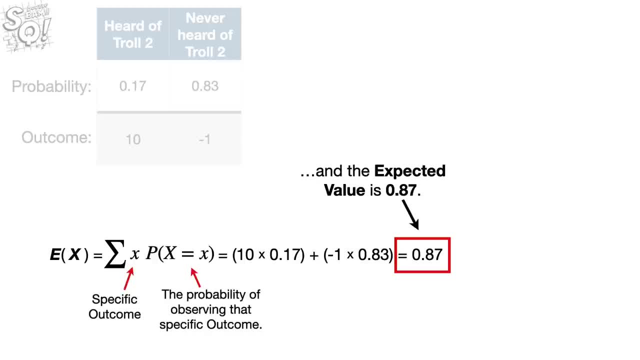 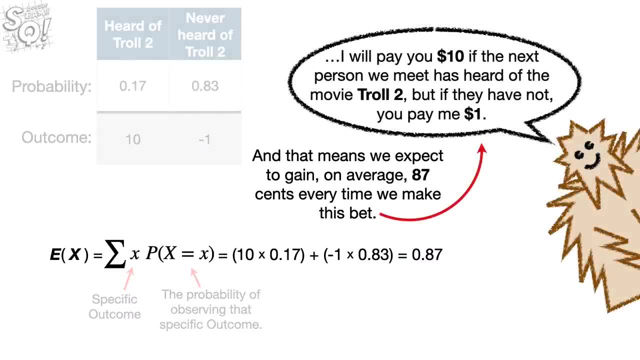 Now we just do the math and the expected value is 0.87.. And that means we expect to gain on average 87 cents every time we make this bet, And that means Statsquatch is the worst gambler ever. 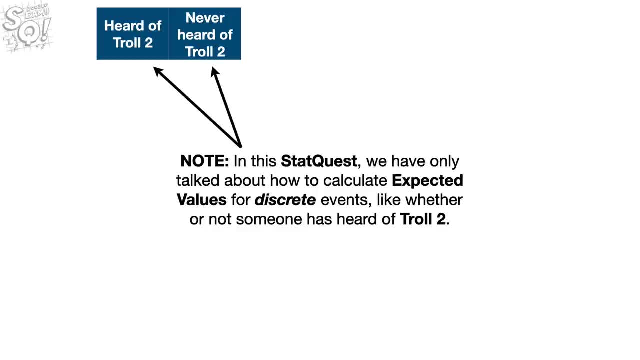 Triple bam. In this stat quest, we have only talked about how to calculate expected values for discrete events, Like whether or not someone is going to be able to get a win, Or whether or not someone is going to be able to get a win. 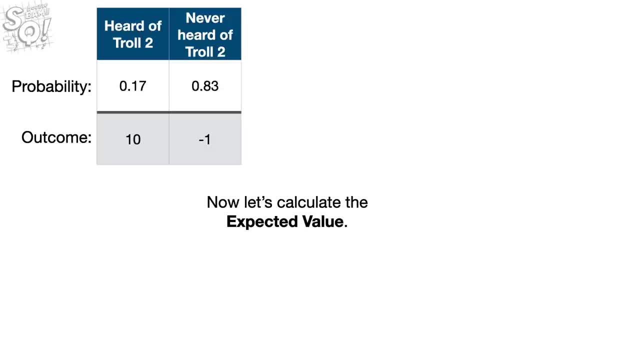 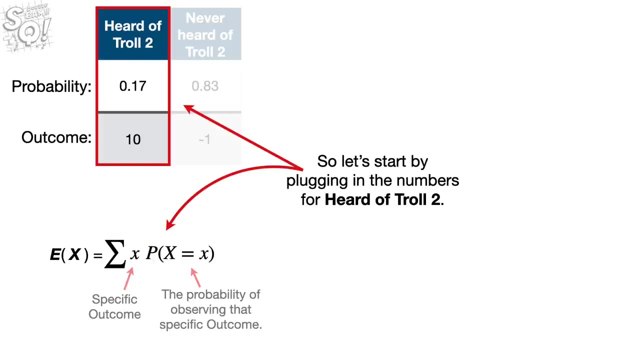 So these are the two outcomes. Now let's calculate the expected value. The expected value is the sum of each outcome times its associated probability. So let's start by plugging in the numbers for Heard of Troll: 2.. First, the outcome X is 10.00.. 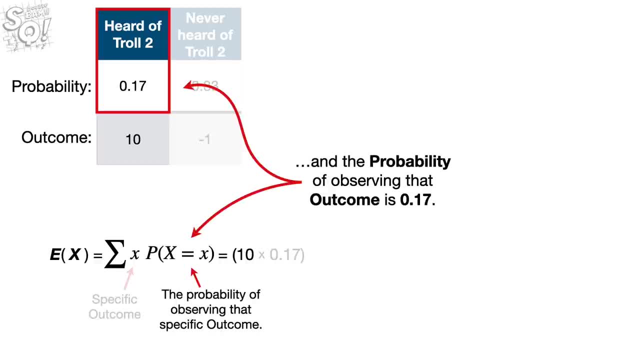 And the outcome X is 10.00.. And the outcome X is 10.00.. And the probability of observing that outcome is 0.17.. Now we add the term for Never Heard of Troll, 2.. The outcome X is negative: 1.. 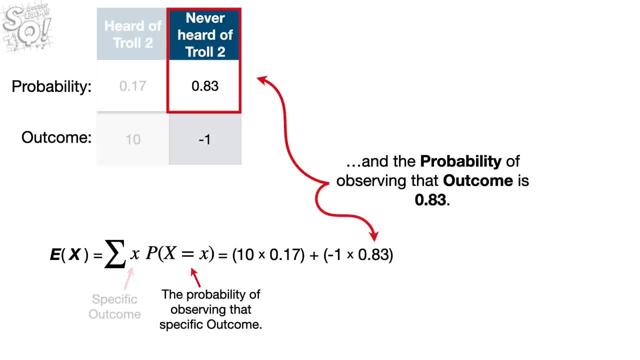 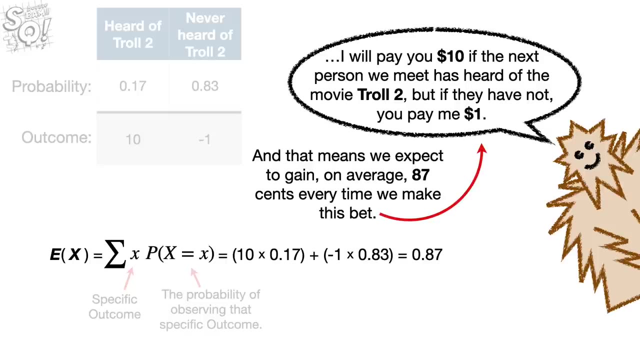 And the probability of observing that outcome is 0.83.. Now we just do the math And the expected value is 0.87. And that means we expect to gain on average $0.87.. And that means we expect to gain on average about $60.. 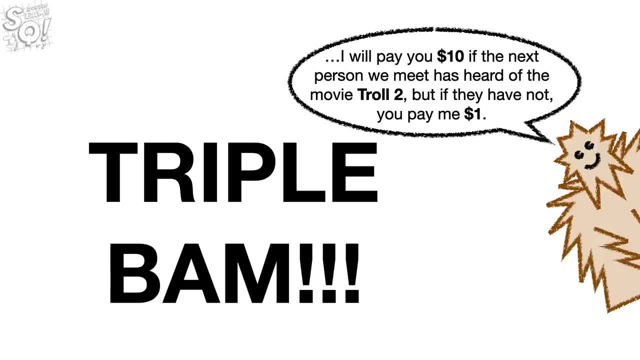 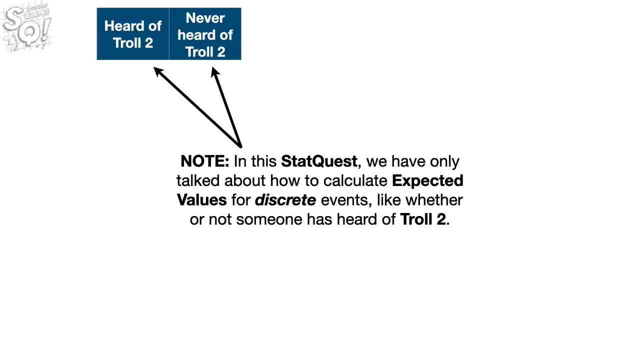 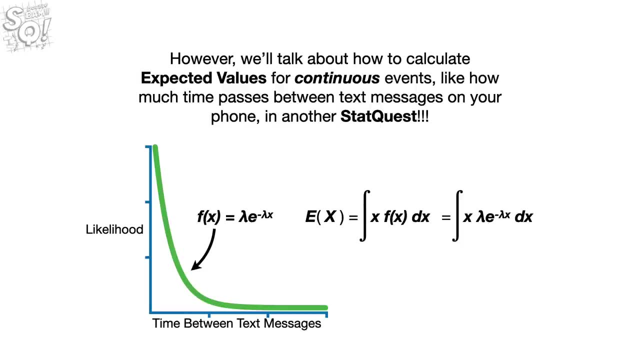 And that means we expect to gain about $80.. So that is the algorithm for使用. the latest code, Trol 2, is thinking about how to use as much data as possible, that is, to estimate the Increasing and decreasing the extension of supply and demand alongside traditional spending. 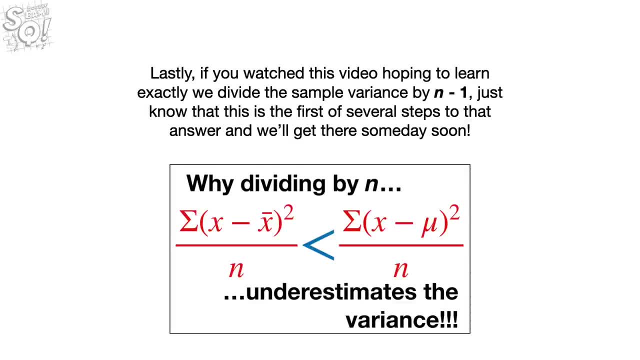 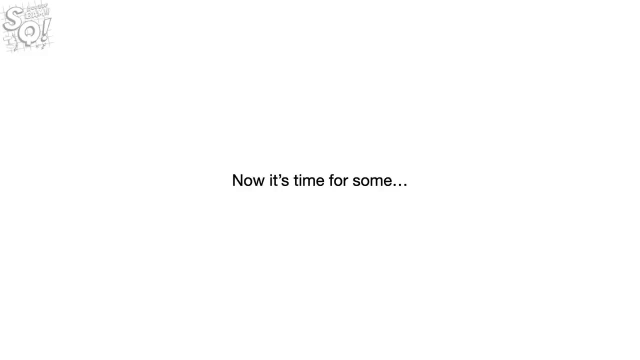 phone in another StatQuest. Lastly, if you watch this video hoping to learn exactly why we divide the sample variance by n minus 1, just know that this is the first of several steps to that answer, and we'll get there someday soon. Now it's time for some shameless self-promotion. 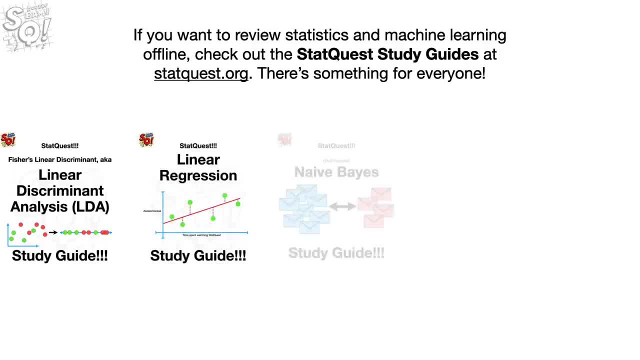 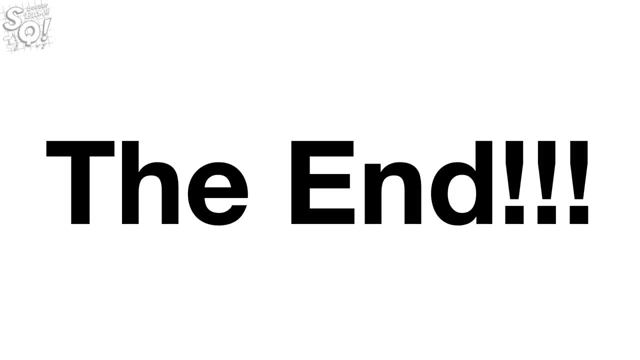 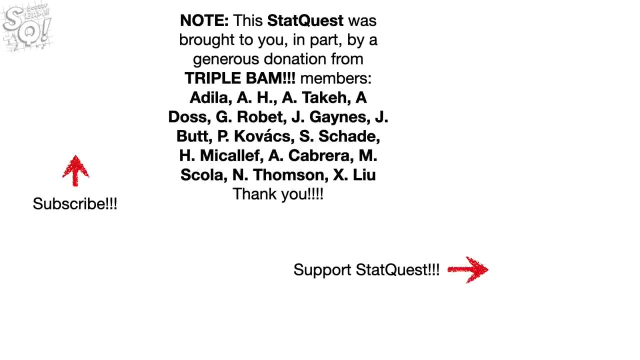 If you want to review statistics and machine learning offline, check out the StatQuest study guides at StatQuestorg. There's something for everyone. Hooray, We've made it to the end of another exciting StatQuest. If you like this StatQuest and want to see more, please subscribe. 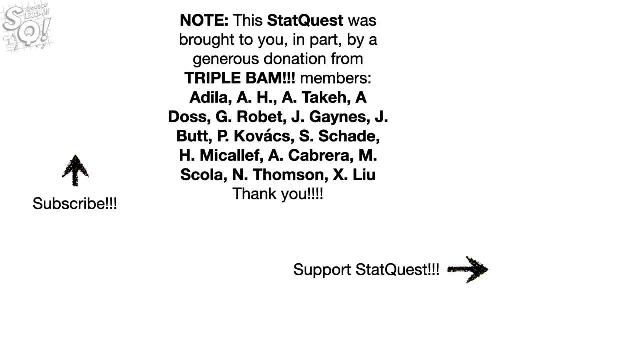 And if you want to support StatQuest, consider contributing to my Patreon campaign, becoming a channel member, buying one or two of my original songs, or a t-shirt or a hoodie, or just donate. The links are in the description below. All right until next time. quest on. Thanks for watching.